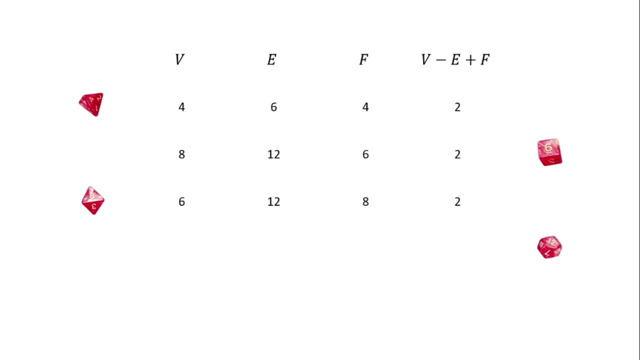 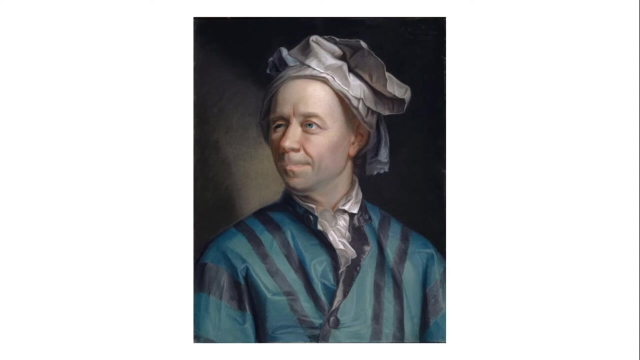 The eight-sided octahedron, the twelve-sided dodecahedron and the critical twenty-sided icosahedron. Euler proved this formula by starting with a polyhedron and removing pieces out of it in succession. He noted that with each removal, the quantity V minus E plus. 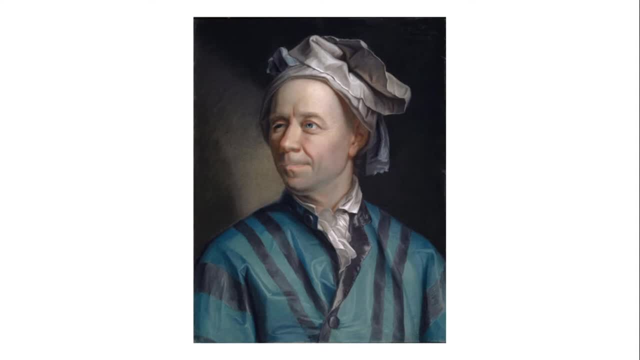 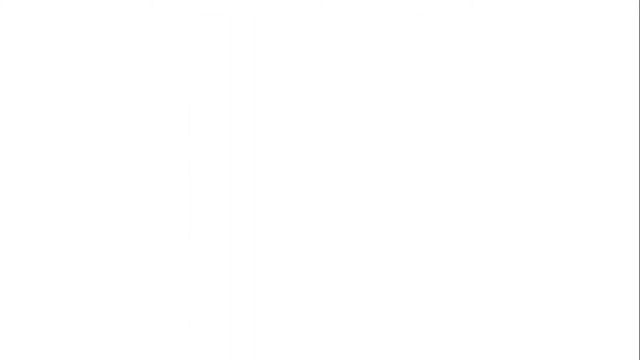 2 would decrease. However, this proof does not answer the last question, as he fails to uncover the deeper connection this innocent-looking equation has with topology. To uncover this connection, I'll follow the proof by French mathematician Adrien-Marie Legendre. This is one of my favorite proofs because it's simple, elegant, ingenious and 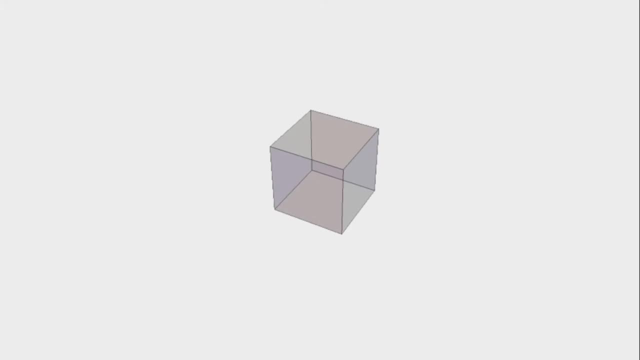 it gives insight into the equation. We start with a polyhedron and we choose a point inside of it. Then we put a polyhedron inside the sphere, with the point chosen coinciding with the center of it. The next step from. 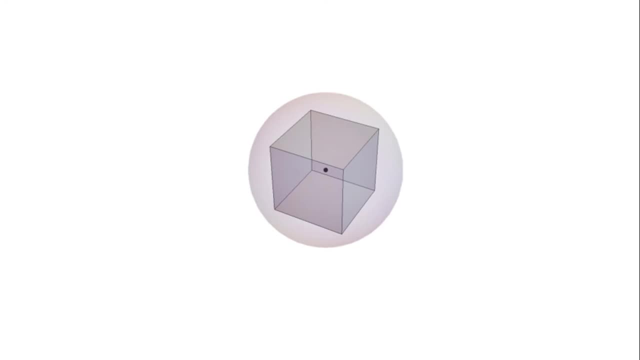 the center. we will project the edges onto the sphere. Just imagine the center of the sphere is a light bulb. then the shadow, the edges cast on the sphere, are exactly the projection, Mathematically for any point in the edge. we connect the center to it and we prolong. the line until we reach the sphere. This is the first step. The second step is to connect the center to the sphere. The third step is to connect the center to the sphere. The third step is to connect the center to the sphere. The fourth step is to connect the center. 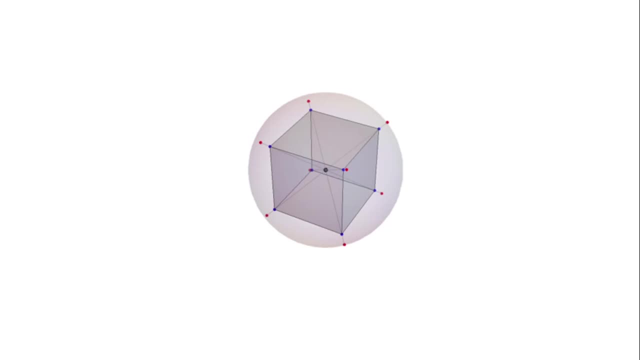 to the sphere And that's the projection of that point. After all the points are projected, we have the projection of the edges on the sphere. With that, we can now forget about the polyhedron and just focus on the sphere Instead of worrying about the many types of polyhedrons. we just reduce the problem to 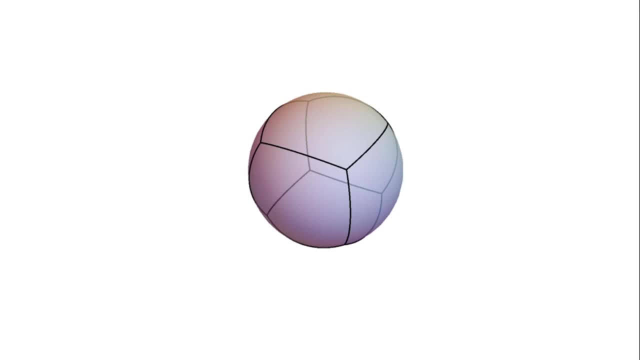 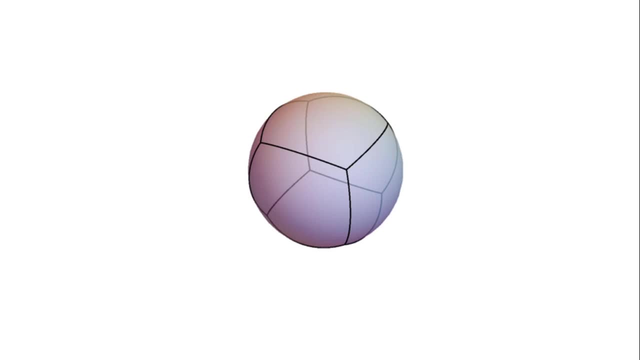 of the sphere is 1.. The radius of the sphere is 1.. The radius of the sphere is 1.. He computed the same quantity in two different ways, In this case the area of the sphere. The easier of the two is to directly apply the formula for the surface area of the sphere. 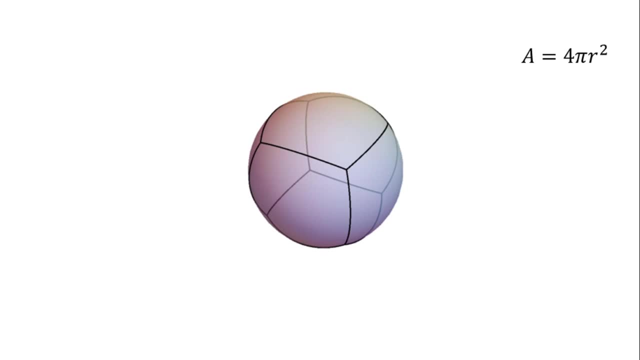 given by 4π times the radius squared, And since the radius is 1, the area is just 4π. The second way is to sum the areas of the several divisions that we made. There's a simple theorem for the area of polygons in a unit sphere. 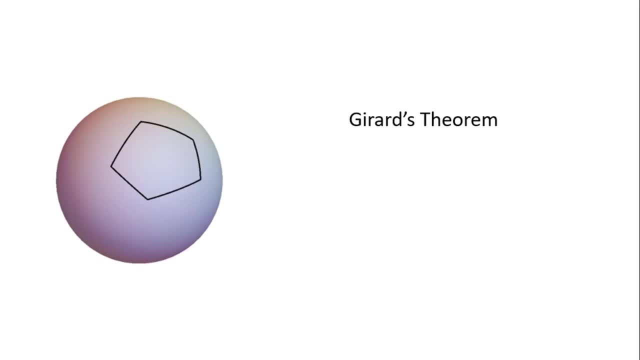 It's called Girard's theorem. It says that the area of n side polygon on a sphere with angles alpha 1 to alpha n is given in radians by the angular excess, And remember that 2 pi radians is equal to 360 degrees. Now, using the distributive law, we get a good way of visualizing this theorem. 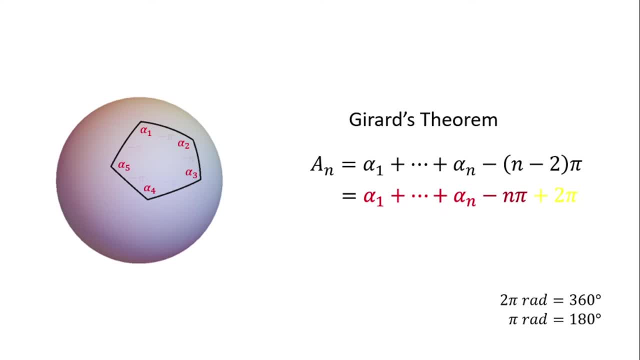 Each vertex contributes its angle to the area, each edge negatively contributes its angle minus pi and the interior contributes to the full angle of 2 pi. Now back to computing the area Using the contribution of each part to the area. the sum of the individual areas is easy to compute. 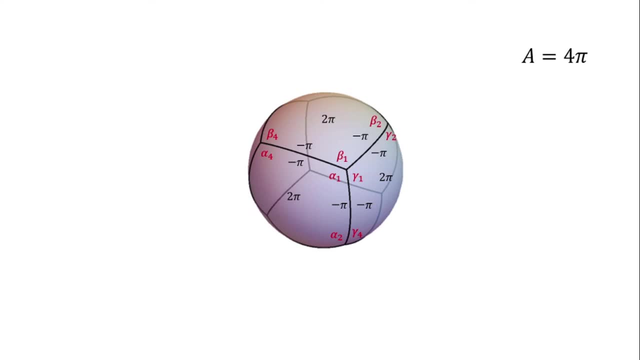 Around each vertex. the angles form a full angle, that is 2 pi radians, and there are only v vertices, so their contribution to the area is 2 pi times v, Approximately 2 v z. übrigens, here are 2 p visits to the syrup point Phoenix. 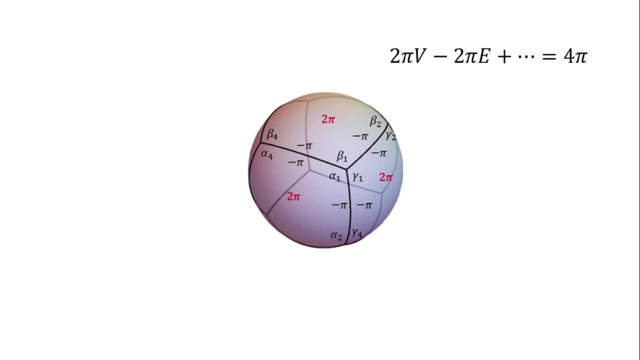 Each edge belongs to 2 faces, so it contributes 2 times with minus pi, for a total contribution of a minus 2 pi times e. Finally, each face contributes with 2 pi to the area totaling a 2 pi times f. contribution to the formula. 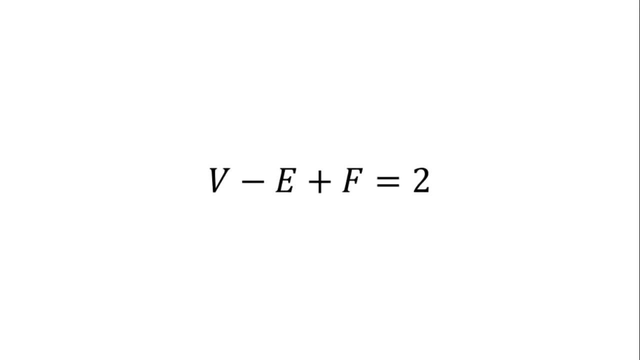 the only thing left to do is dividing both sides by 2 pi to get the euler formula for the polyhedra shows that every decomposition of a sphere satisfies this formula. And the reason polyhedra satisfy it is because, in a sense, 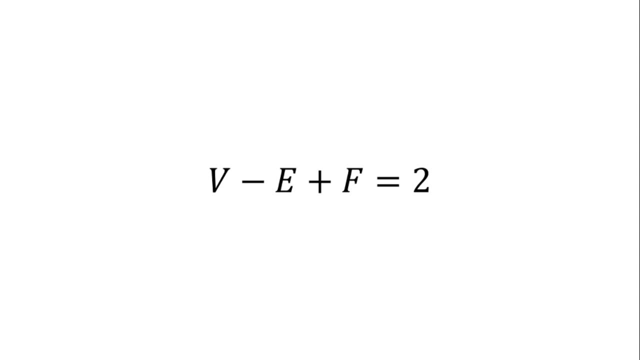 they can be molded and transformed into a sphere. For example, a projection is one of those waves, And in mathematics we'd say that they are topologically the same as a sphere. I hope you found this as interesting as I did when I first read about it. 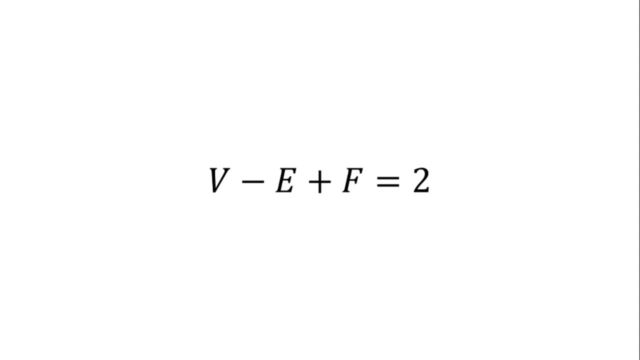 I made this video for 3Blue1Brown- the Summer of Math Exposition. Thank you for listening.